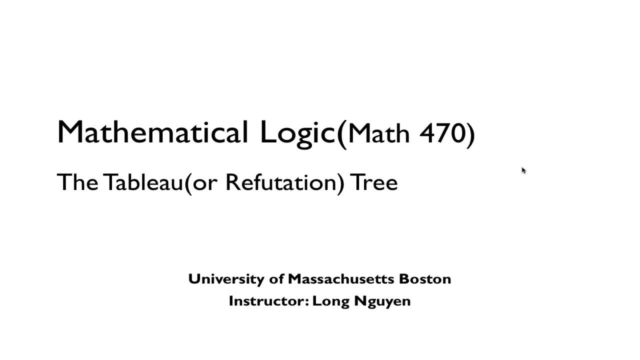 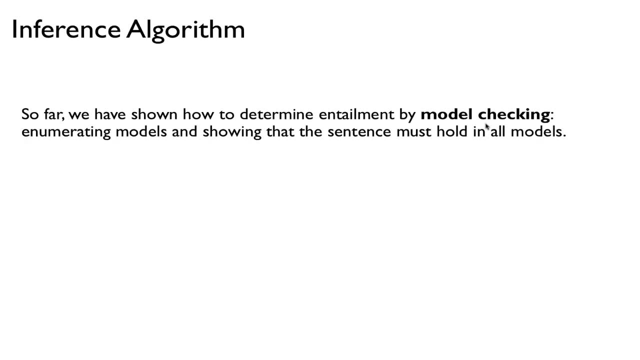 Hi, welcome back to Mathematical Logic. We're going to talk about the tableau tree, or the refutation tree in this video. So far we have shown how to determine entailment or logical implication by model checking, Basically enumerating all possible models or looking at all the rows of the true table and then checking to see which of those assignments satisfy the implication. 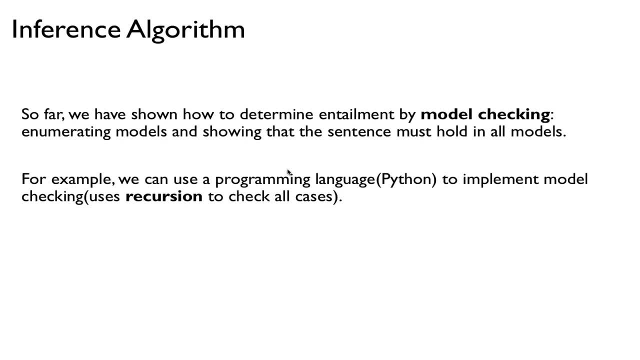 For example, you can use a language like Python to implement model checking, For example. it turns out that you use recursion to basically check all possible cases. It's just a brute force approach, But model checking is an example of an inference algorithm. 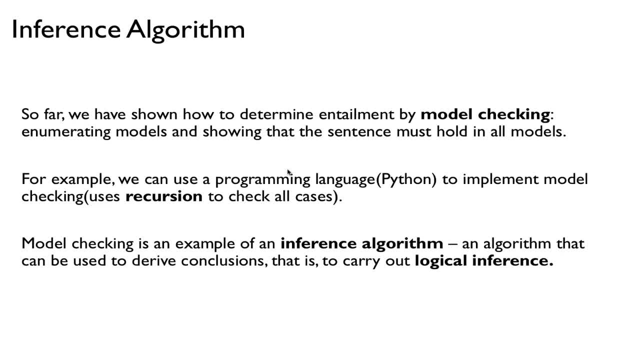 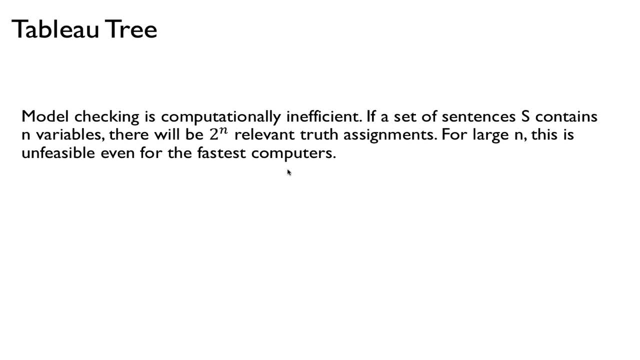 It's an algorithm that can be used to derive conclusions or to carry out logical inference. We saw that in the last few videos. Model checking, however, is actually not very efficient If you have a set of senses and it contains n variables or n symbols. 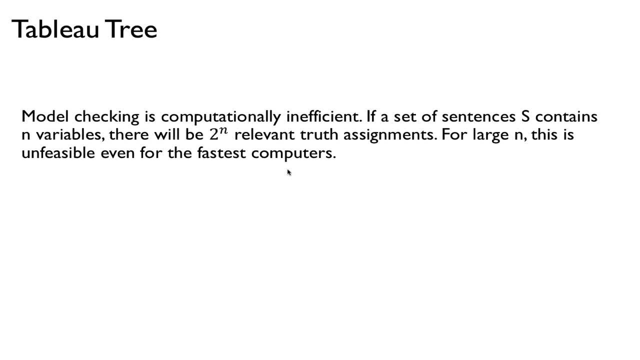 then there will be 2 to the n relevant truth assignments, or 2 to the n rows of the truth table, And so for large n, this is exponential, And so this is not even possible for even the fastest computers. So in this video, in this lecture, we're going to talk more about a more efficient method of doing this. 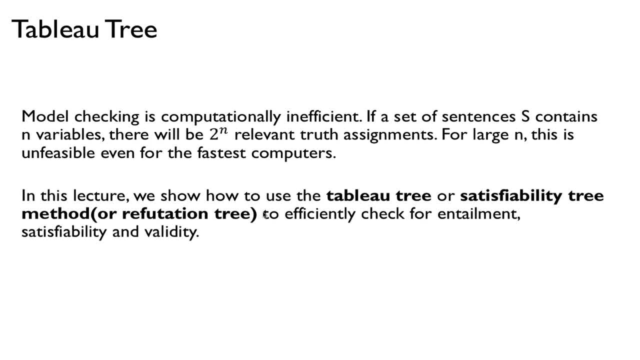 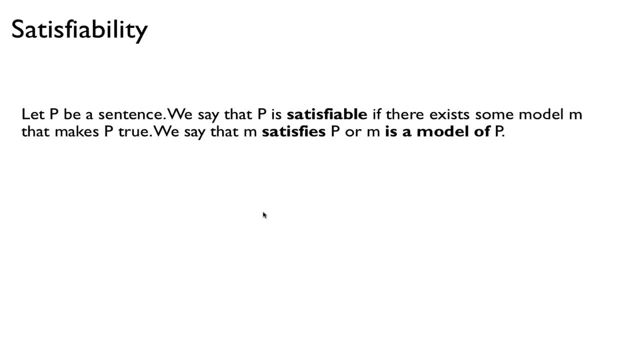 And we're going to talk about how to use a tree, a refutation tree, to check for entailment, for satisfiability and for validity. So let's actually first begin by reviewing some of these terms. If p is a sentence, then we say that p is satisfiable if we can find a model m that makes p true. 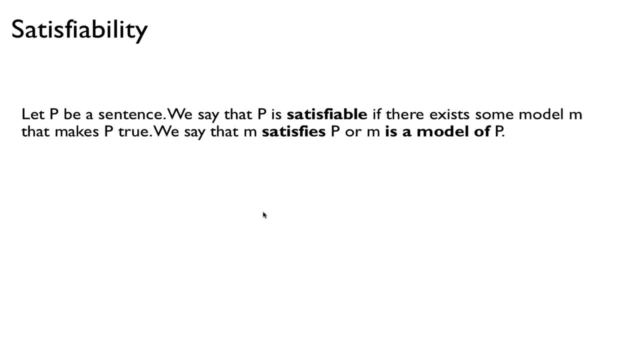 We can find an assignment or a model that makes the sentence true And then that assignment is a model of p. If you have a bunch of senses- s1 to sn- then we say that the set s is satisfiable if we can find a model that satisfies all senses. 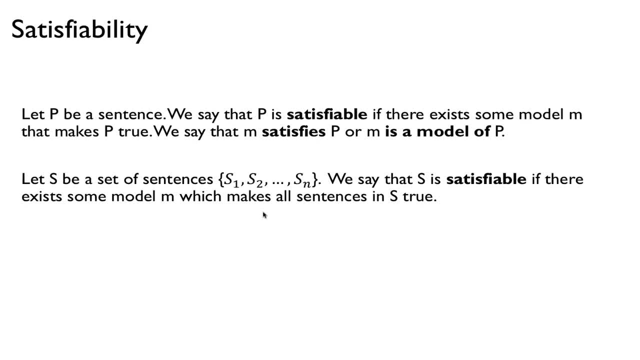 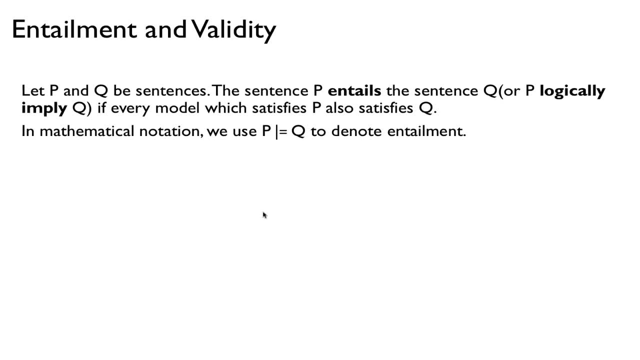 All senses in s make all of them true. If you have p and q are senses, then p entails q or p logically implies q, If every model that satisfies p also satisfies q, And we use this notation to denote entailment. And then, in general, if you have a set of senses- s1 to sn- 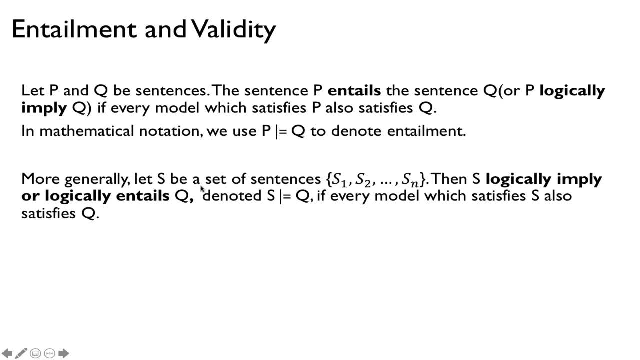 then that set s largely implies or largely entails q, If every model that satisfies all of s will also satisfy q. And finally, a sentence is valid: if it's true in all models, It's true in all, and another way of saying this is that: 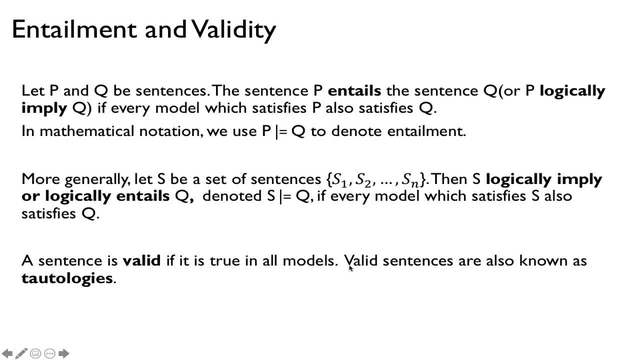 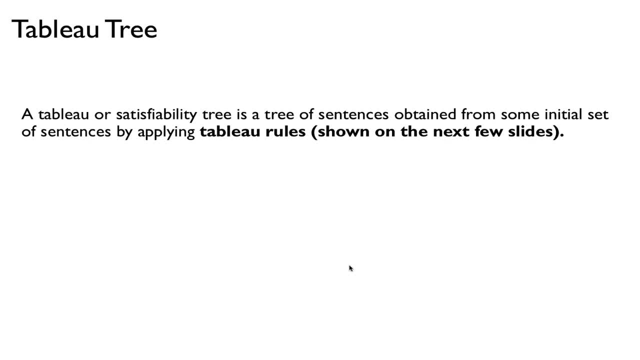 tautology is a valid sentence. Okay, so those are just review. Let's talk about this tableau tree or this satisfiability tree. It's basically a tree of senses obtained from some initial set of senses by applying a tableau rule. It's a set of rules that we'll see in a moment. 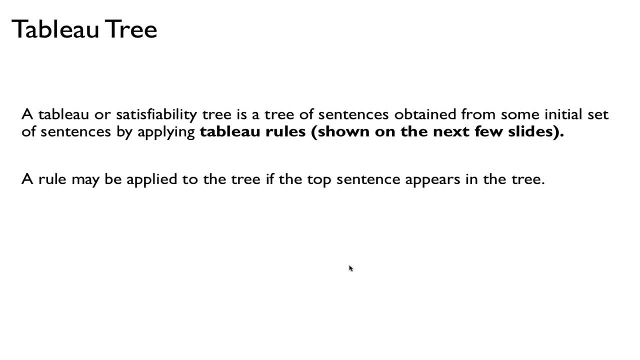 And the idea is that a rule can be applied to the tree if the top sentence of the rule appears in the tree And the idea is that you can create these branches. that goes down And to apply a rule, we add a branch or branches at the bottom of the rule. 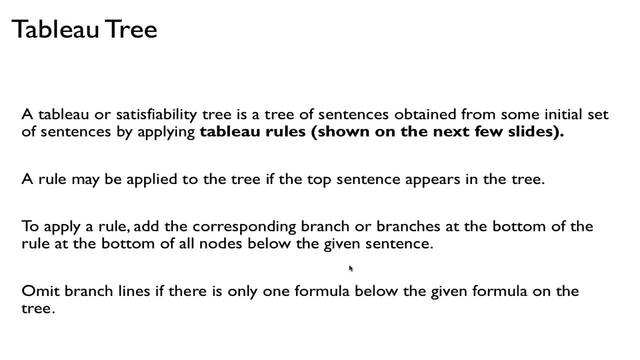 below the given sentence, And then we're also going to emit branch lines if there's only one formula below the given formula. So we'll make sense of that in a moment. So let's kind of see some of these rules and see how this will work. 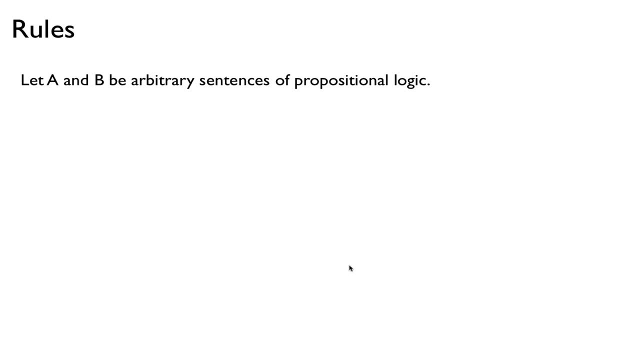 Suppose you have a and b senses in propositional logic. So here's the first rule: You have a or b. If that's the sentence in the tree, we can branch out into a or b, And that makes sense, because an or means that there's two paths. 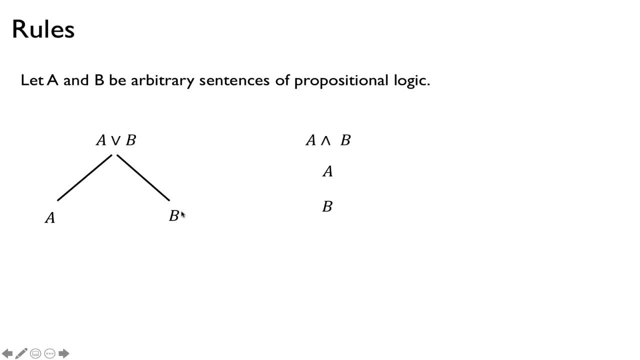 either this way or the other way. a and b means that both a and b has to be true, so there's no branching. It's the same path. We write a and b separately to denote a and b. So these rules are actually very obvious why they work. 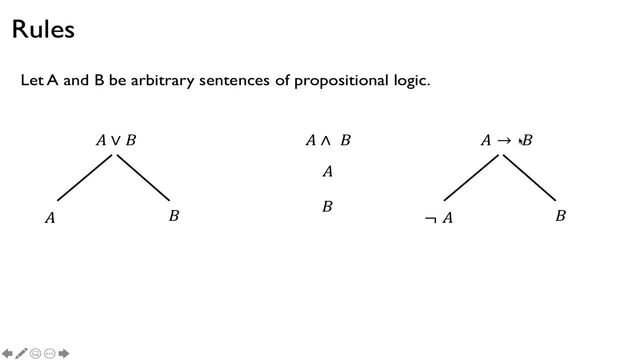 And then a implies b means. remember, in one of the homework we proved that a implies b is actually equivalent to not a or b, And so if you have this in the tree, we can break it down into these components. The goal here is that we have these rules. 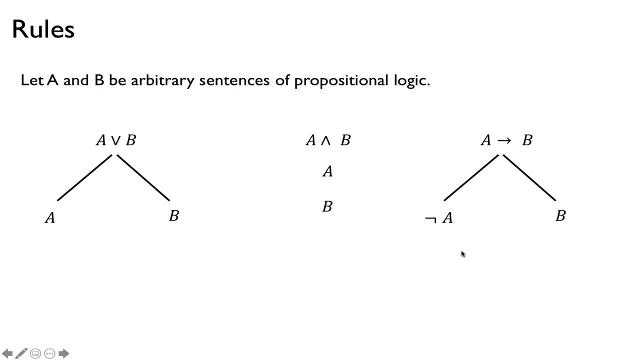 that we're trying to break down into atomic senses, simple senses, and then we can use that to find counterexamples or to prove something. So those are three rules. Here's three more Now. these are the negation rules. Same thing as before, but now we're negating everything. 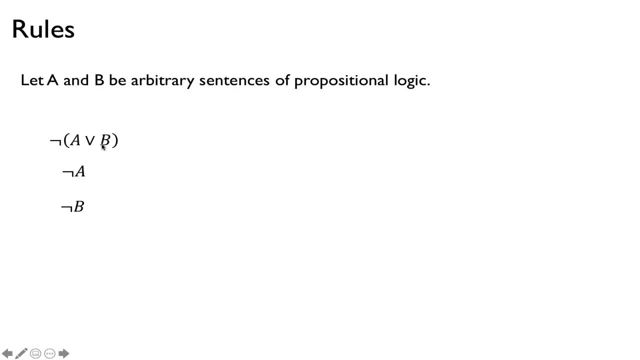 So not a or b. So remember that from the previous video, the Morgan's Laws, we can actually bring in the not so that this becomes not a and not b. So this simplifies to not a or b And then not a and b becomes not a or not b. 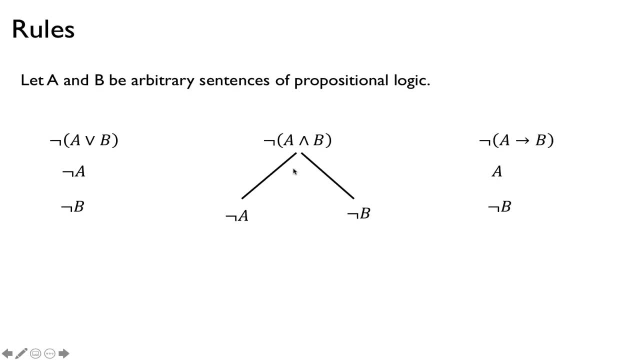 So we have that branching. So these basically come from the previous three. And finally, the inside of this is not a or b, So the Morgan's Law will make this a and not b. So there's that. So that's how you resolve that rule. 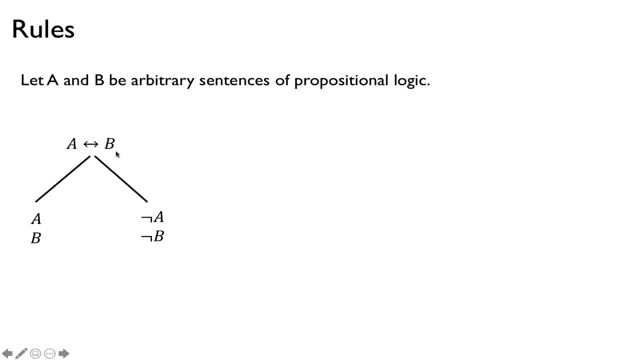 So here's the last three rules. Biconditional, So a if and only if, b means that either they're both the same- Well, that means that they're both the same, So either they're both true or both false. 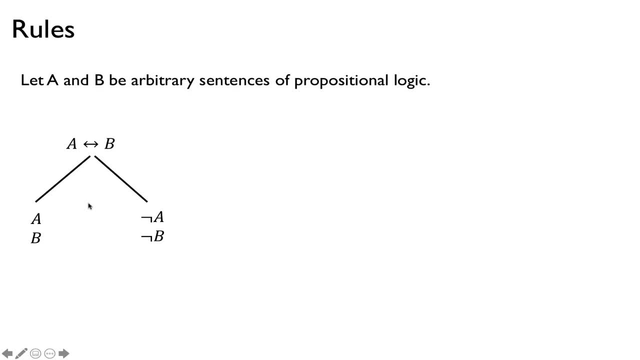 So a- b here means they're both true, Not a and not b means they're both false. In either case, we have biconditional, And so these definitely are a little more complicated And you basically want to memorize all these rules. 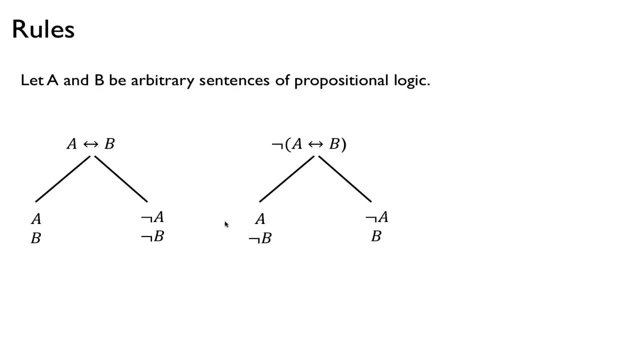 I mean, there's no way to do this without understanding and memorizing these rules. And finally, we're to negate the by conditional if it's not true that they're equivalent. that means that either a and not b, or not a and b. 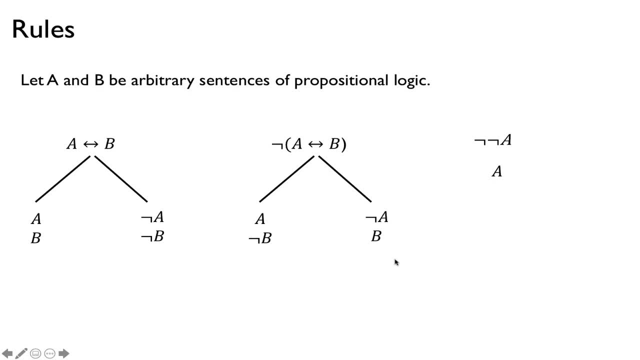 And finally, the double negation rule says that not, not a is a. Yeah, those are the nine rules that we have to memorize and help us basically again break down these connectives into smaller components. Okay, a branch of a tree is a path to the tree. 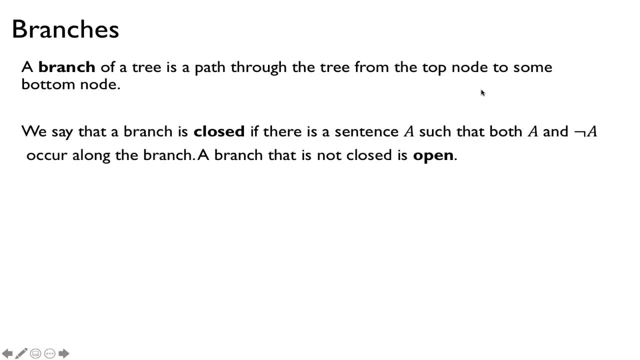 from the top node to some bottom node. We say that a branch is closed If there's a sentence, a, such that both a and not a occur along the same branch. And a branch is open if it is not closed. So it's closed if you have a and it's a negation. 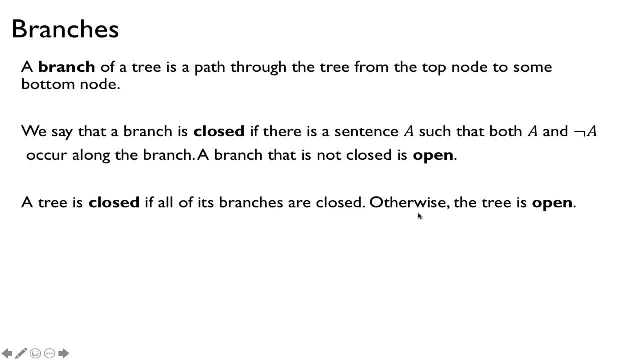 And the tree is closed if all the branches are closed. Otherwise the tree is open. So the idea here is that branches correspond to attempts to build a model satisfying the senses along the path, in particular the senses at the very top, And then a closed branch corresponds to an attempt. 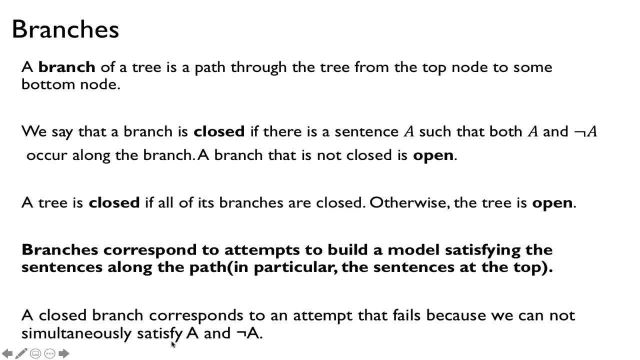 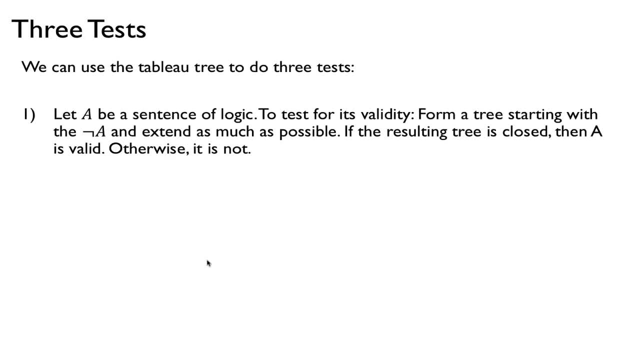 that fails because we cannot simultaneously satisfy a and not a. So let's kind of see an example. I think the example will clarify all of this. Well, first of all, we're going to use the tree to do one of three tests. 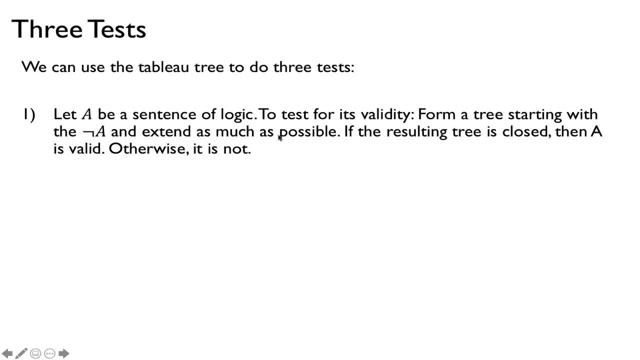 The first test is: we want to know whether a certain sentence is a tautology or a certain sentence is valid. So to test for validity, we form a tree, starting with, not a. We want to know if a is always true. You remember, in one of the previous videos. 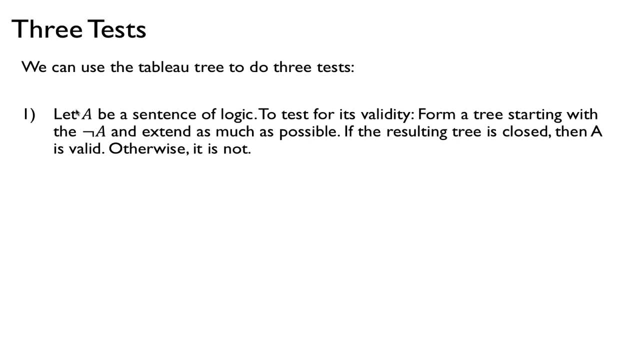 we showed that a is tautology by doing a proof by contradiction. So this is like that We start out. we want to prove that a is always true. Well, start out by assuming that a is false, so not a, And we're going to extend the tree as much as possible. 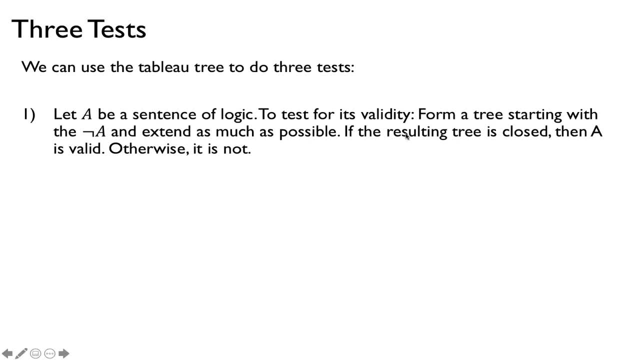 applying all those rules, And if the resulting tree is closed, then a is valid. Otherwise it is not valid. So again, if the tree is closed, that means that all the paths. so we assume that a is not valid. We assume that a is not true. 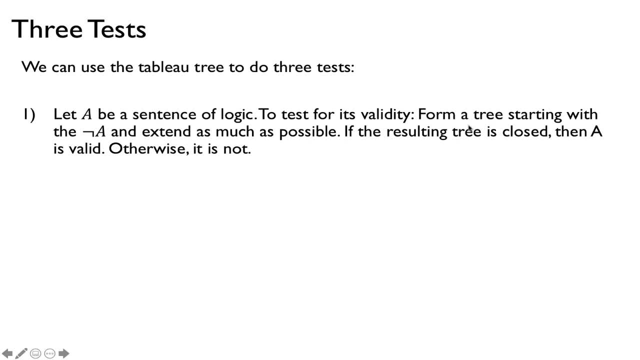 and we found out that all of our paths, we have contradiction in all of our paths, All of our paths give us a and not a, or a sentence and its negation, And so our attempt to show that a is false is not correct. 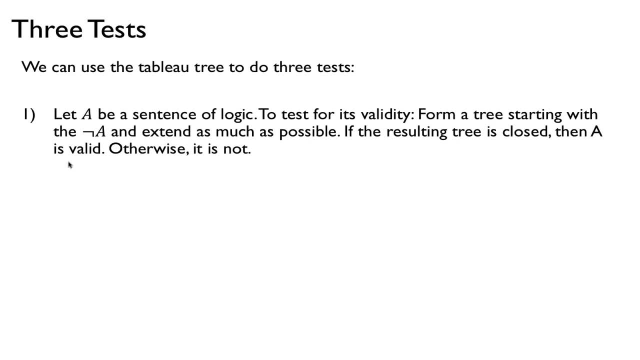 Therefore a must be valid. And then to show entailment. again, it's supposed to have a set of sentences. We want to show that s entails q. Then we form a tree starting with s1,, s2, all the way to sn. 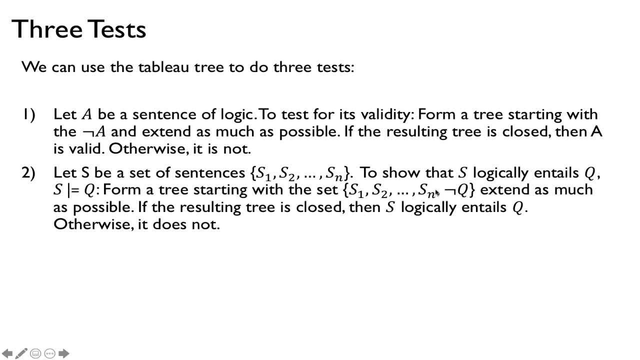 and not q. So basically assume of s1 to sn and then also assume the negation of our conclusion. Then we extend the tree as much as possible And if the tree is closed then s does entail q. The reason is because our attempt to show that 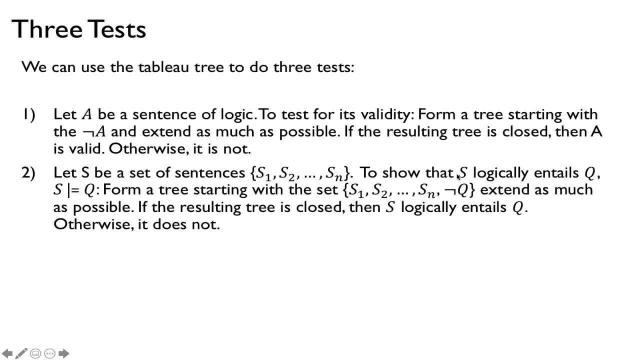 assuming all these assumptions and the negation of the conclusion, we failed that attempt, and so, therefore, we must have entailment. Otherwise, if the tree is open, then we don't have entailment, And then, finally, the last thing we can do with trees is that. 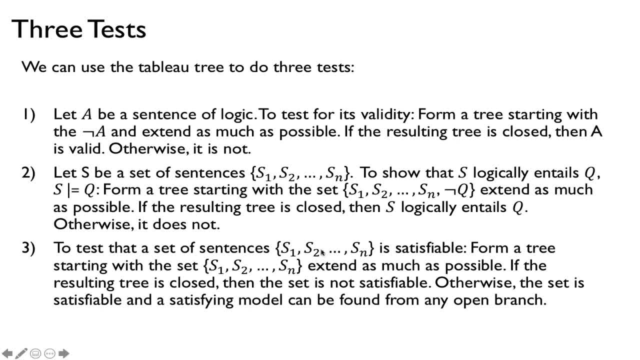 we want to show satisfiability, So you have a bunch of sentences. We want to show that all of these can be satisfied by some model. So we form a tree with all of these And notice here, in this case this is different than the previous case. 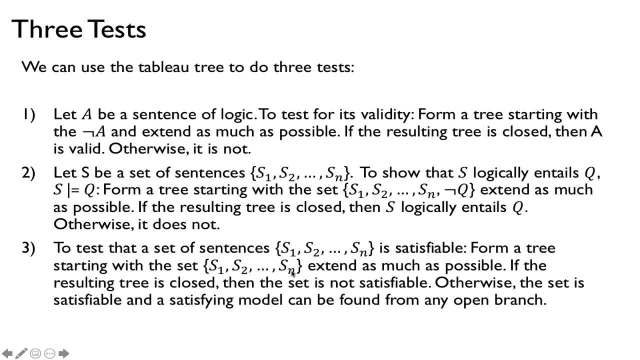 There's no negation here. We start a tree with all these sentences, Extend as much as possible. If the resulting tree is closed, then the set s is not satisfiable, because we cannot find a model that makes this true. Otherwise, the tree is open. 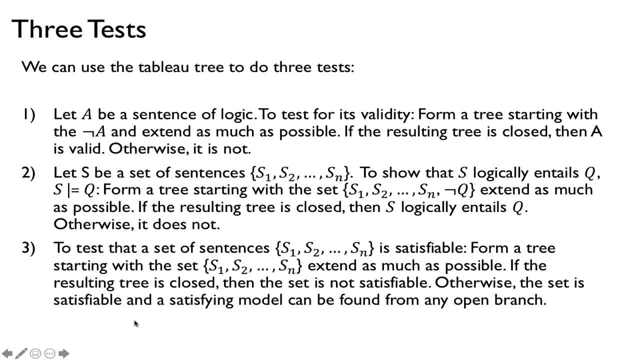 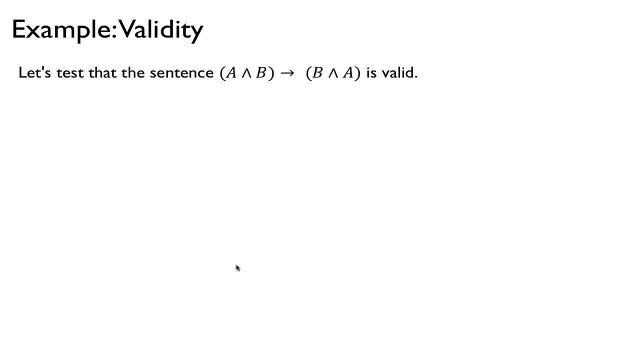 and we have at least one open branch, then that branch will help us satisfy this set. Okay, let's actually see some examples, So let's do the first one. This is the first test. We want to prove that this is valid. 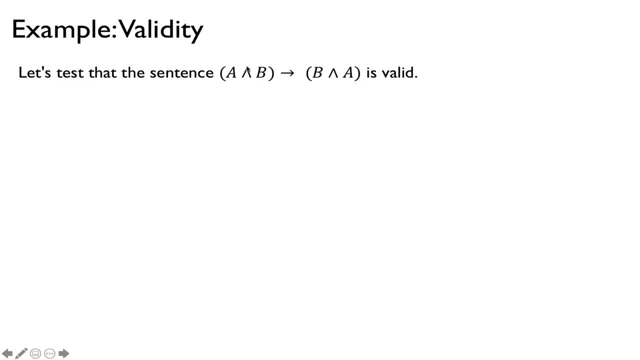 meaning. this is always true And that makes sense, because a and b implies b and a. This is always going to be true for any assignment of a and b for any model. So we want to show that this is a tautology. 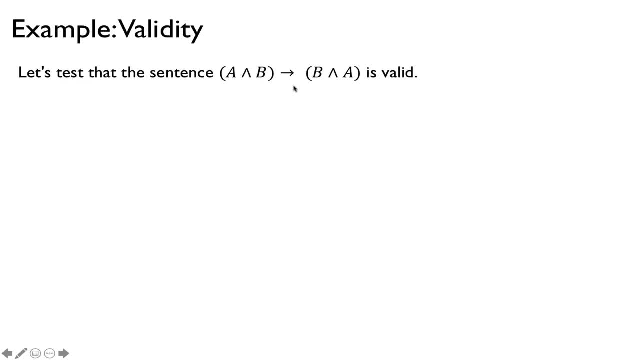 Okay to do that. we take it and we're going to assume that it's false. So we're going to negate this. So here's the first. Here's the root of the tree. It's that negation of what we want to prove. 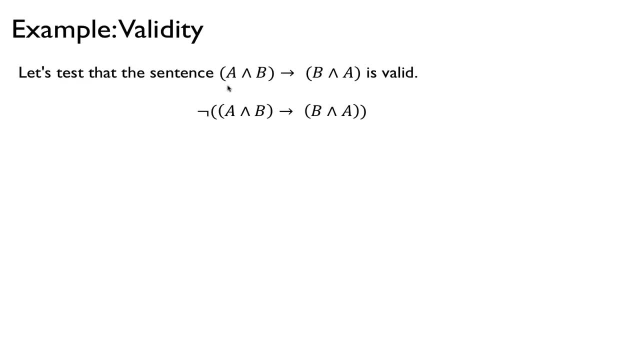 And now we're going to apply the rules to simplify this. So this is a conditional and this is a negation. So we apply one of the rules, We're going to say that. So, remember, the conditional is not Well, if I call this x and this y, 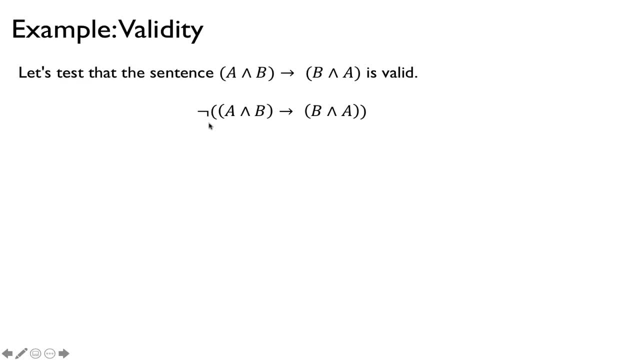 conditional says that not x or y, And so when I negate that, then I get x and not y. So I'm going to resolve this by saying this and not that. So, again, this is one of the nine rules that we saw. 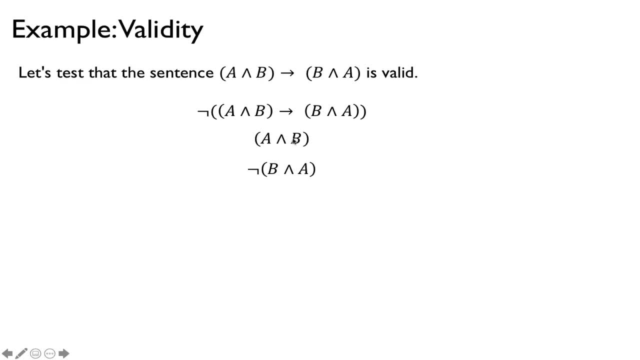 So what this does is that we replace this sentence with an equivalent representation in this one branch here And so now we don't really need this. We actually resolved this already, So this is equivalent to this information. So I'm going to cross this out. 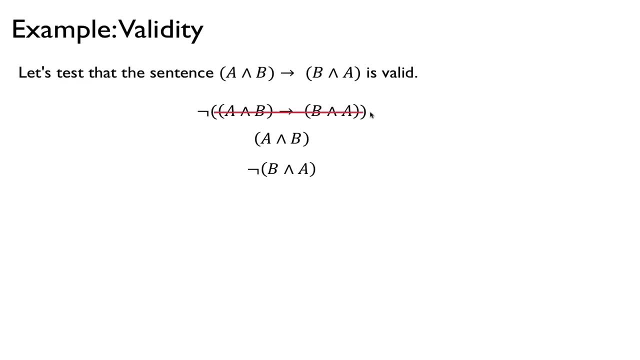 just so that we know that we already resolved that sentence. So now, so this tree is still the same tree. We just throw away some redundant information. Now let's try to resolve one of these. We won't eventually resolve both, but let's resolve, say, this one, the top one. 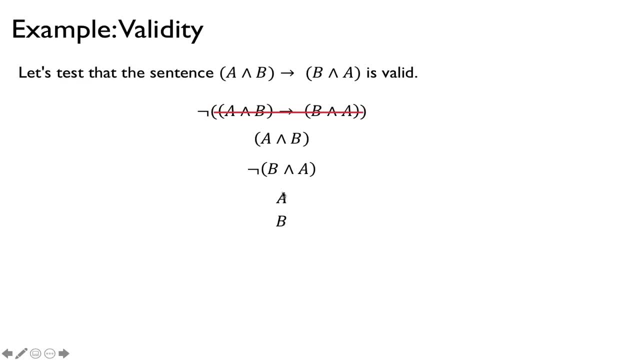 So this is a and b. so one of the rules says that is, you write a and b along. here Again, I resolve it. so I'm going to cross it out And to resolve this, apply the Morgan's Law, not b or not a. 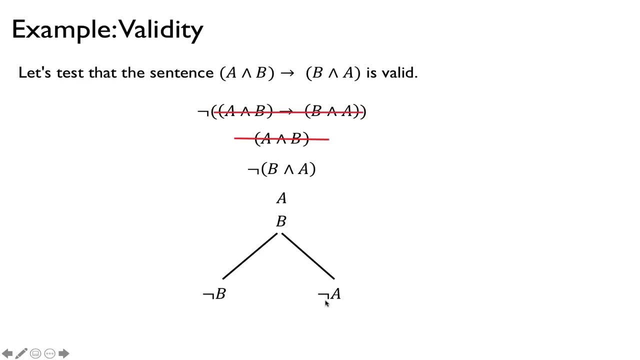 so that's a branching. So not b or not a. So I also want to cross that out too. So again, this is the tree now. Notice now, all the complicated sentences are now very simple. So we have this path: a and b. 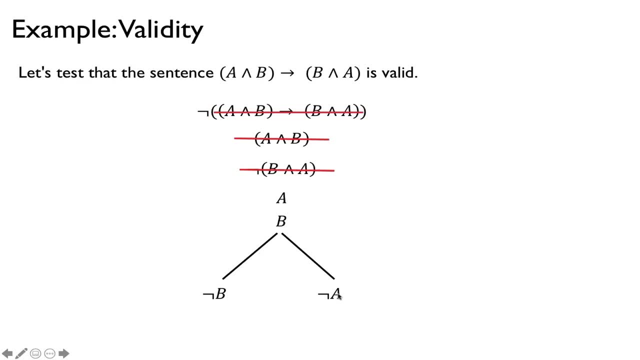 or this path: a and b and not a, So we have two paths there. Notice, both these paths are closed because we have in this b and not b. that's a contradiction. and then a and not a, So we have found a contradiction. 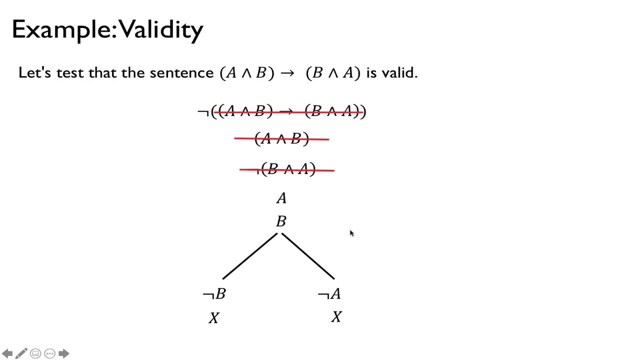 and so these branches are closed, The whole tree is closed. Therefore, we do have that. the sentence is valid. Let's do entailment. We want to show that, given these two assumptions or two sentences, we do imply or entail this sentence. 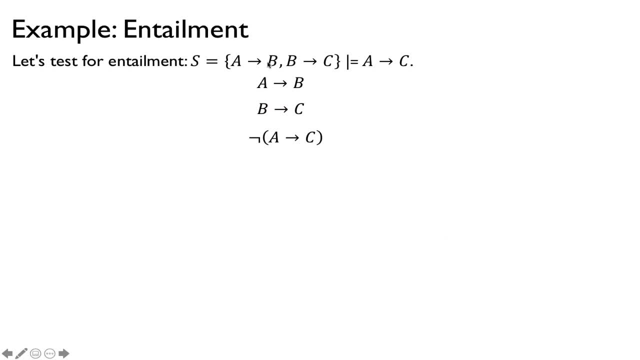 That makes sense because, look at this: a implies b and b implies c. Well, together that should show that a implies c. So that's what we want to show here: logical implication or entailment. So the way we do this, 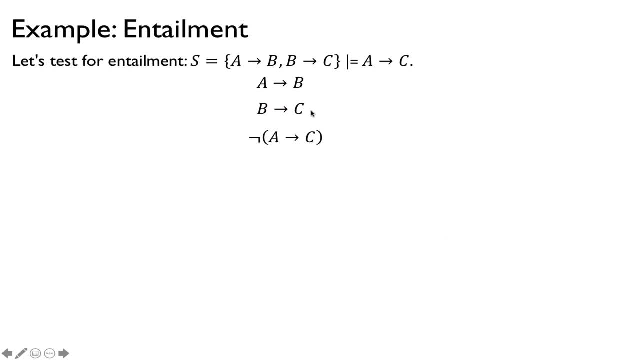 we're going to assume the s, so a implies b and b implies c, and assume the negation of the conclusion. We want to conclude this, so we're going to negate it. We're going to do a contradiction. We want to say: well, assume these. 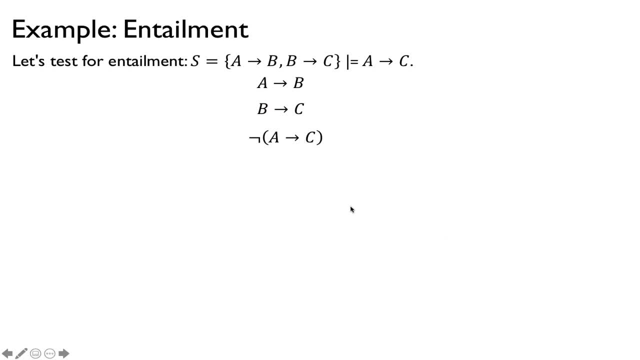 Let's assume that the conclusion is false and see if we can close this tree and get a contradiction. Therefore, the conclusion must be true. So now, these are all of our assumptions. so let's now resolve each of the sentences. The first sentence: this is not a or b. 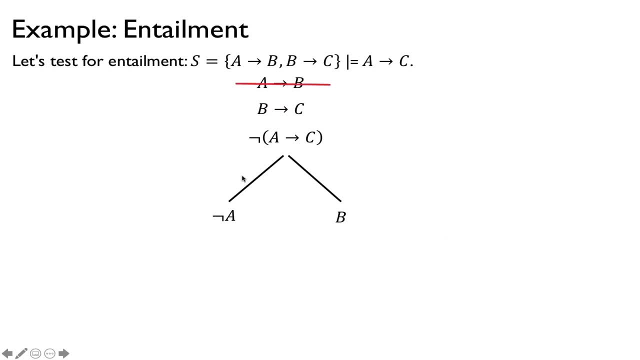 so I branch out and I cross out the top. Then I'm going to resolve this one. This is not b or c, so I have to do that for both of the branches. Not b or c, not b or c. I cross out that sentence. 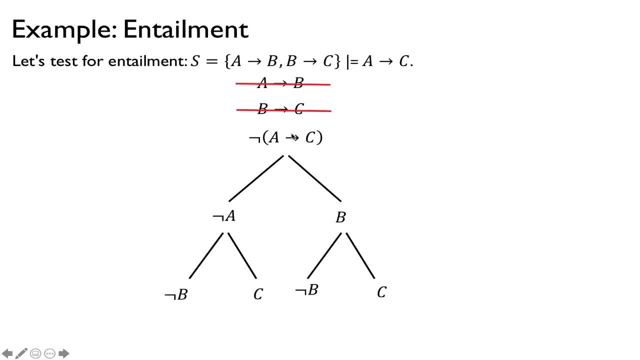 And to resolve this one, this is an or not a or c. so if I apply the Morgan's Law, it would be a and not c. So there's a and not c along all those paths. And notice, now we have some closure here. 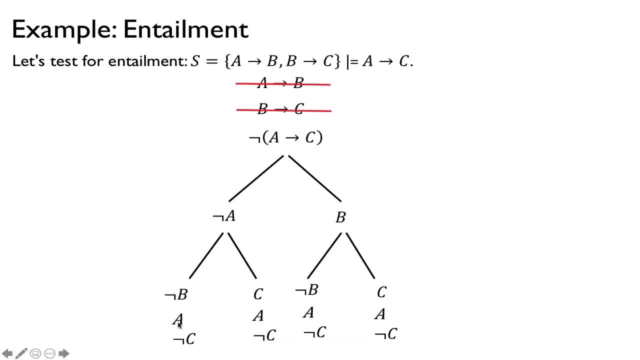 because notice, in this path not a and a, this path a and not a, this path b, b and not c, this path c and not c, So we can actually close all of these paths. So that means this tree is closed. 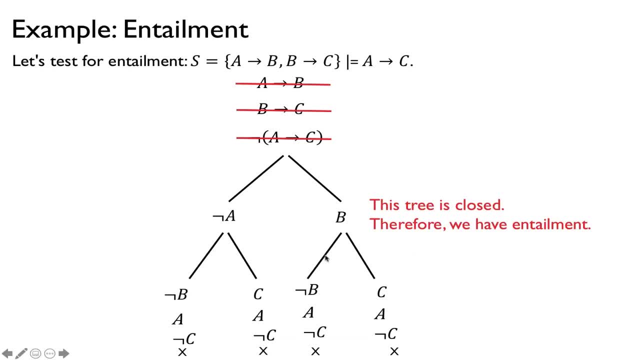 and we do have entailment, By the way, at this point, right here, this is b and not b, so we could actually have stopped that branch. We don't have to finish that branch because there's already a contradiction earlier, but that's fine. 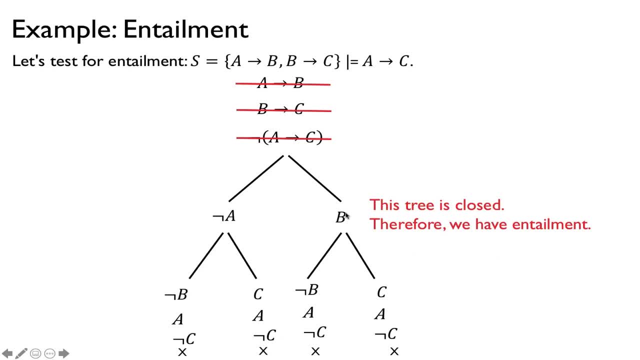 In fact we're going to see an example now that we can actually close things early. If we can close some things early, we don't have to finish that branch. So we're going to redo this problem, except that we're going to do it in a different order. 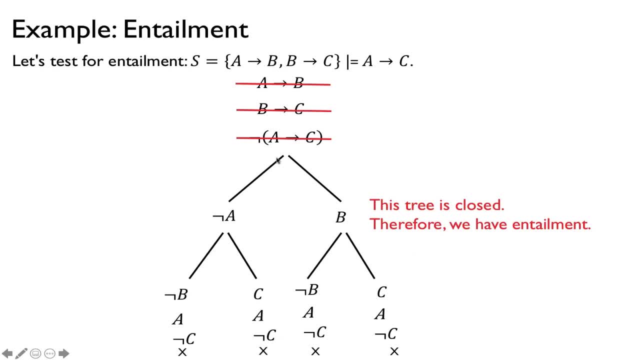 So it doesn't matter what order we do, but sometimes some order is better. So it turns out that it's actually better to do. notice that we did the branching first, all the branching first, and then the non-branching, But it turns out that it would be better. 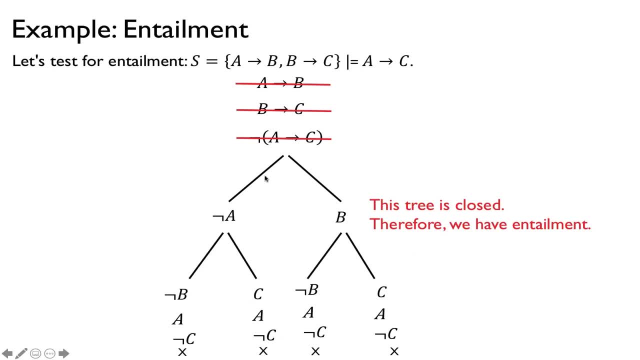 to do the non-branching first. that way we can simplify our tree a little bit. So let's see how that works. So I'm going to do the same problem, but now I'm going to do the non-branching factors first. 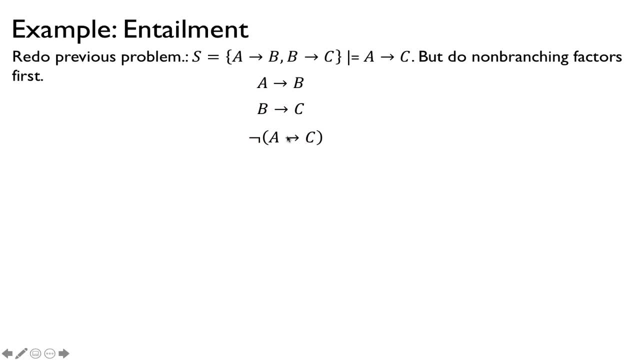 So again you have o and n. we want to do the n first so that we don't have so many branches. So instead of doing the top two, we're going to do this one, resolve this first. So this is going to be a and not c. 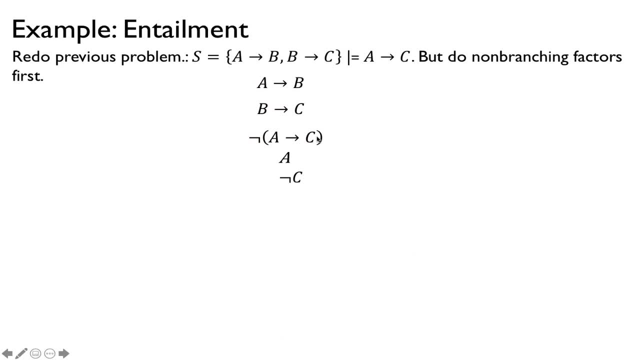 So I'm going to resolve the non-branching factor here, close that, and then now we're going to resolve the branching factors, So not a or b, and then here in this case- by the way, we notice here that this branch is already closed- 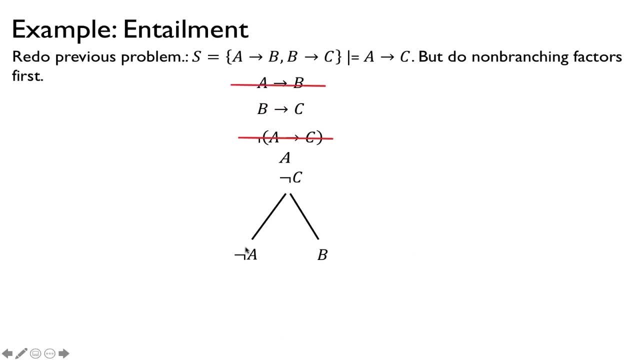 a and not c, so I can actually let me close it. by the way, let's cross it off first and then then I want to close this branch, because there's already a contradiction here, And now I want to resolve this by doing. 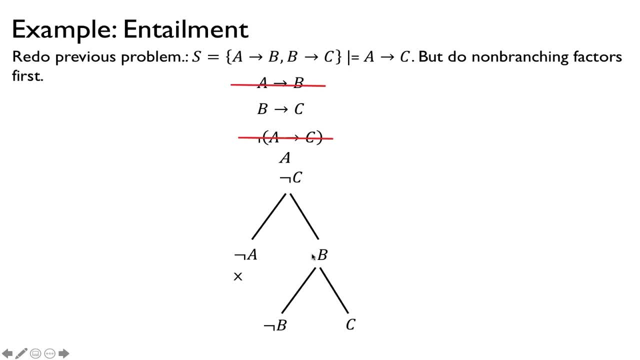 now I'm going to branch. this way I don't have to look at this branch anymore. so if I do that, then I get not b or c And then notice these paths are also closed and so this tree is. notice, this tree is a little bit simpler than the previous tree. 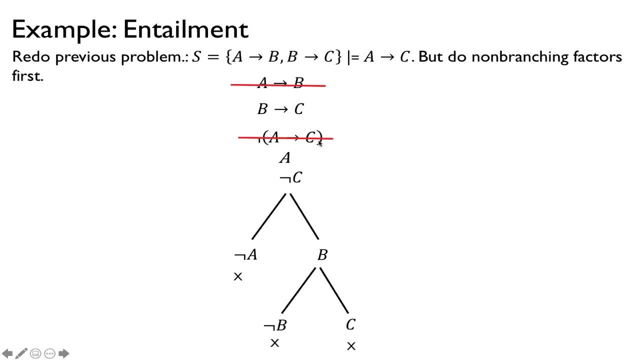 because we did the non-branching factors first. So the tree is closed. therefore, we do have entailment And in the final example we're going to talk about, we're going to figure out how to satisfy a sentence. So here's a sentence. 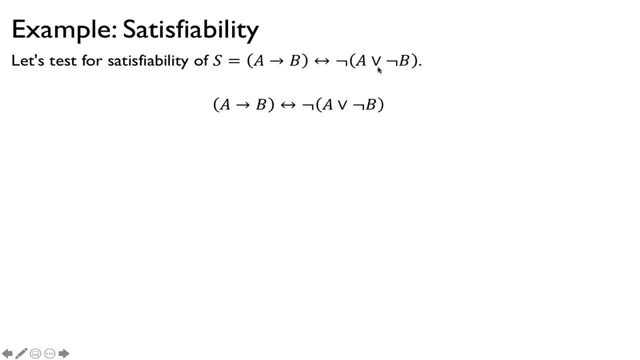 we want to show whether we want to see whether this is satisfiable, In other words, can we find an assignment that makes this true? So, to show satisfiability, we just keep the sentence the same, just like that, and try to extend and apply the rules. 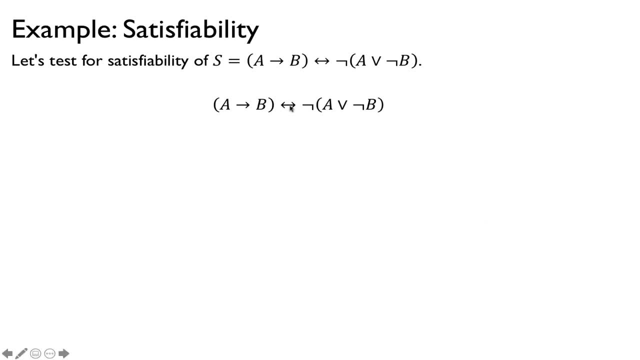 And so this is a biconditional. so we, in one branch we keep them the same, and in the other branch we negate both of them. So that's the biconditional rule. So I crossed out the top. 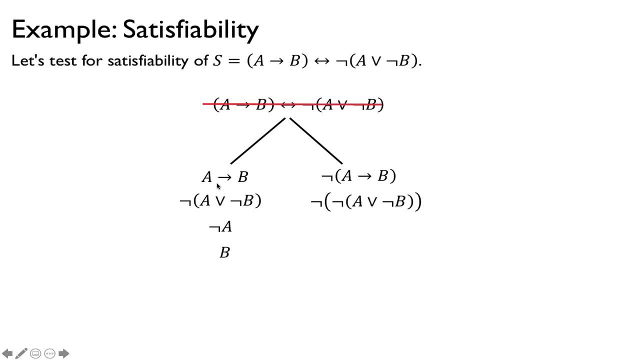 and now I'm going to resolve each of these. So let's do this one. I want to do again: non-branching factor first. So De Morgan's Law says that this should be not a and b, So I do that. 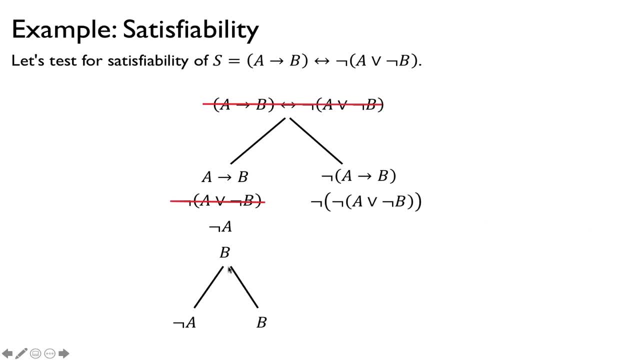 and I cross this out, And then I'm going to finish this by doing not a or b Cross that out. So I basically resolve the left side here And notice that I have, on the left side at least, I've resolved everything. 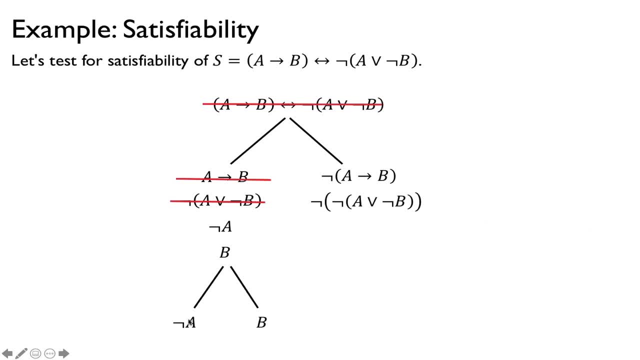 So everything is now atomic. But notice, there's no contradiction along this. So these are open branches. So that means that we found a way to satisfy the original sentence. So, again, an open branch is a way to satisfy it. So we actually have two ways here.